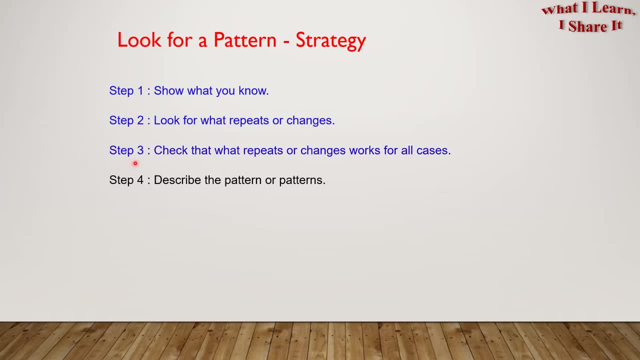 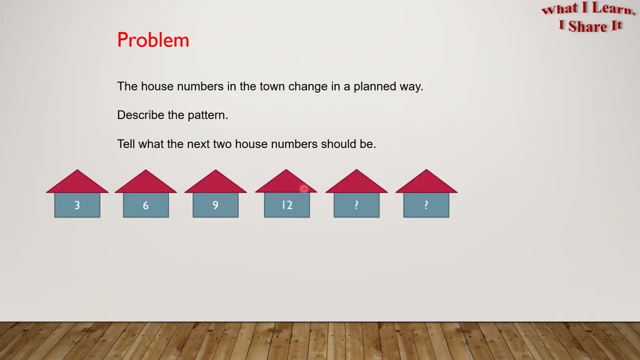 Step 3. Check that what repeats or changes works for all cases. Step 4. Describe the pattern or patterns. Here is a problem. to help us understand the strategy, The house numbers in the town change in a planned way. Describe the pattern. 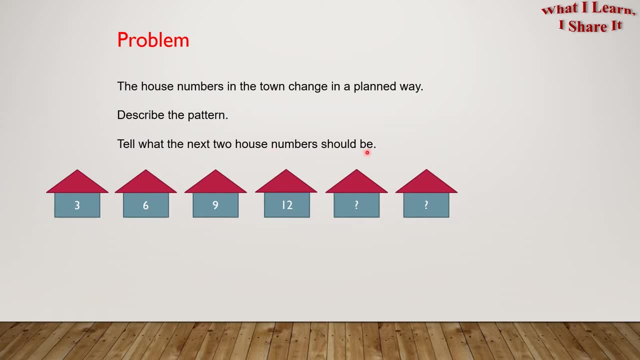 Tell what the next, What the next two house numbers should be. So here are the houses and their numbers on them. Do you want to try it yourself? Feel free to pause the video and try it yourself. Do you want to see how I solved it? 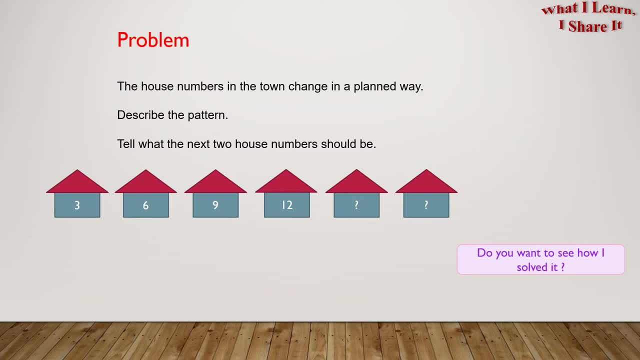 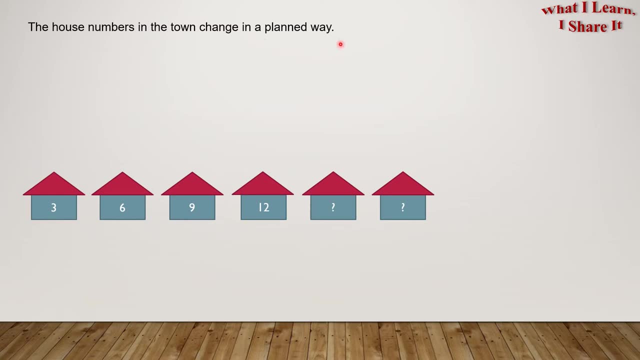 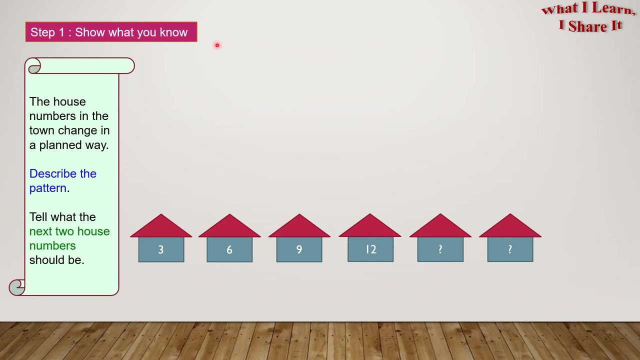 I solved it in a step by step way. Let's see it. The house numbers in the town change in a planned way. Look for what repeats or changes. Describe the pattern. Tell what the next two house numbers should be. Step 1. Show what you know. 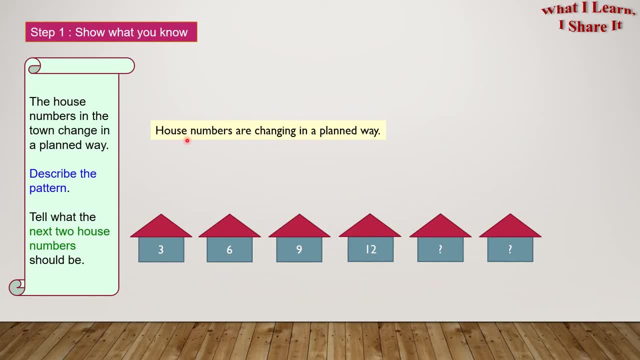 So what do we know? We know that the house numbers are changing in a planned way. Step 2. Look for what repeats or changes. Look for what repeats or changes. Put it on the surfaces. So what do we know? changes, so what repeats or what changes in this pattern the house numbers are? 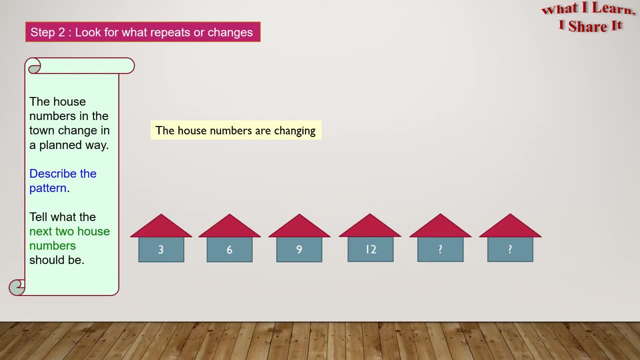 changing. step 3: check that what repeats or changes works for all cases. yes, all the house numbers are changing. in fact, all the house numbers are increasing in the same pattern, so they're increasing on the same pattern. step 4: describe the pattern or patterns. so what is the pattern? the house numbers are multiples. 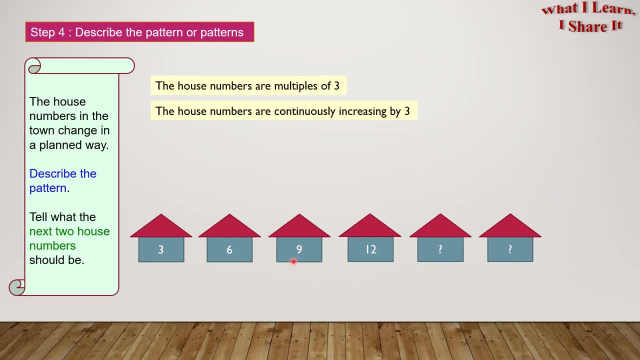 of 3 and the house numbers are continuously increasing by 3, so the pattern is times 3 or plus 3. let's use the times 3 over here. so I've labeled these houses like with 1, 2, 3, 4, 5, 6. so 3 times 1 is 3, 3 times 2 is 6, 3. 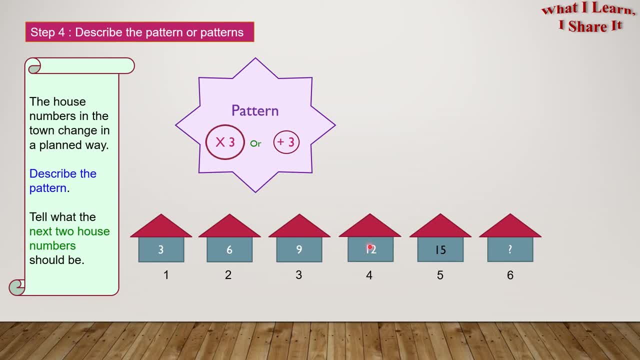 times 3 is 9, 3 times 4 is 12, 3 times 5 is 15. and what is 6? yes, it's 18. the next two house numbers will be 15 and 18, so use the addition strategy now: 3 plus 3. 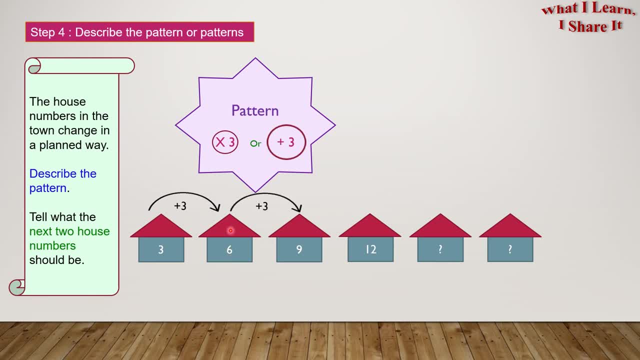 is 6, 6 plus 3 is 9, 9 plus 3 is 12, 12 plus 3 is 15 and 15 plus 3 is 18. so 15 and 15 plus 3 is 18. so 15 and 15 plus 3 is 8 is 2 and 18, so 6 plus 2 is 8. so if I growing up, I'm 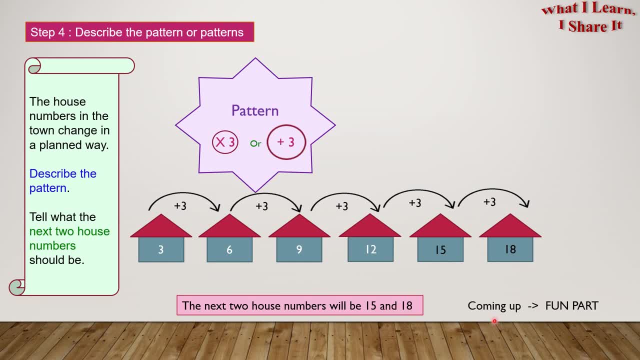 going to take the plus one and take the 2 home times 1, and take the 2 home times 2 times 2 will be 1, 3 times 4 plus 3 and 1 and 3, 2, 3 times 4 and then 5 times 5 and. 6. it makes 1. at the same, 77, 7 and 9, 8. the plus 2 will be 3, 7 and 6, 3, 4 and 2. 3 is in fact 7 and 3, 9 in a bunch. here are some examples to help. 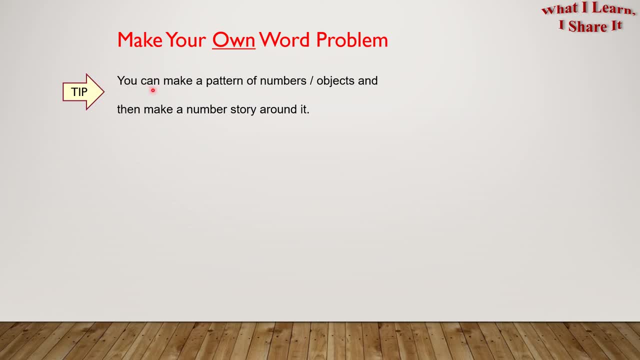 you with this pattern until number 2, and here is an example. make your own word problem. here is a tip: you need to stop 5 coins on day 2, and 7 coins on day 3, and so on. How many coins will he save on day 4 and day 5??